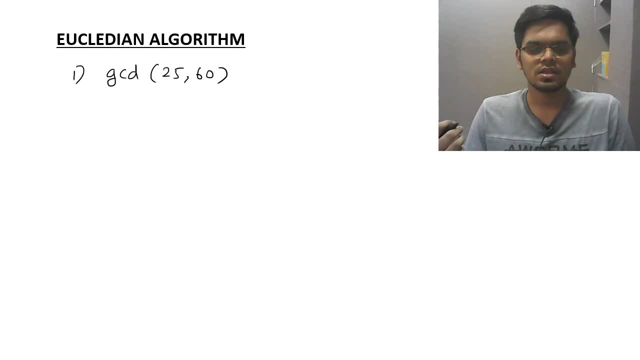 various methods. Once I will show you method 1, then we can see the shortcut also. So how to solve this quotient using Euclidean? We have to make a table. In that table we have four columns. Column 1 is quotient, Column 2 is R1, which is the greatest number between the two, and column 3 is 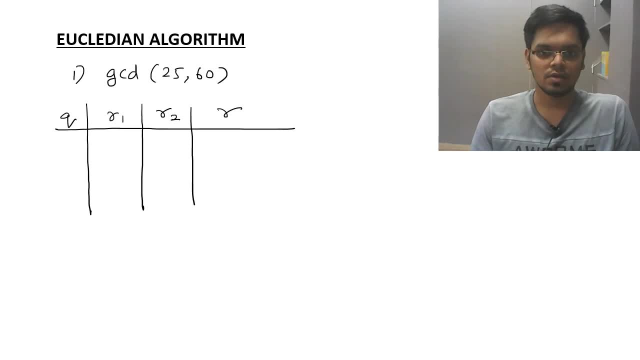 R2.. Column 4: it is the remainder, which is R. So I guess the first step is clear, that is, making the table. We have to write four columns: Column 1 is quotient, Column 2 is row 1.. Column 3 is R2 and column 4 is R. Now, this R1 is the greatest value among these two, Which is: 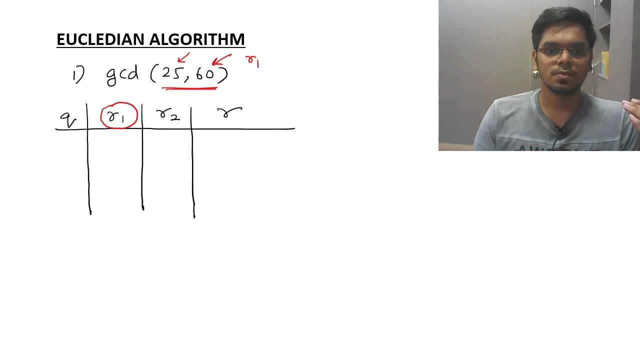 greatest, 60 is greatest right. So this would be R1.. The remaining part would be R2.. So I will write 60 first, then R2. here Now how to find quotient and remainder. It is very simple. Basic calculation: 60 is divided by 25.. So 25 twos are, it would be 50 and remainder would be 10.. So the numerator part. 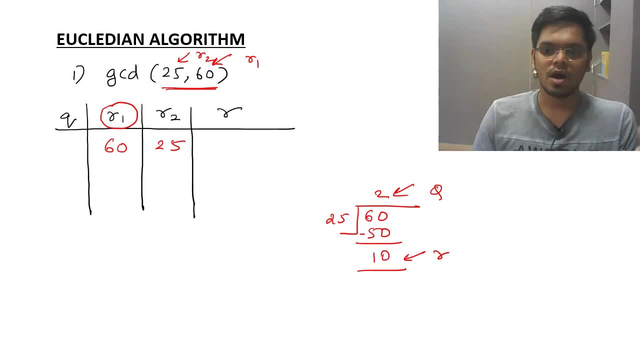 the denominator part is the remainder part. I hope you know how to do the basic division. So quotient is 2.. Remainder is 10.. Now comes the next step, Very important step In the next step: how to get R1 and R2? We have to shift the position. R2 would be here and R would be here. We are shifting. 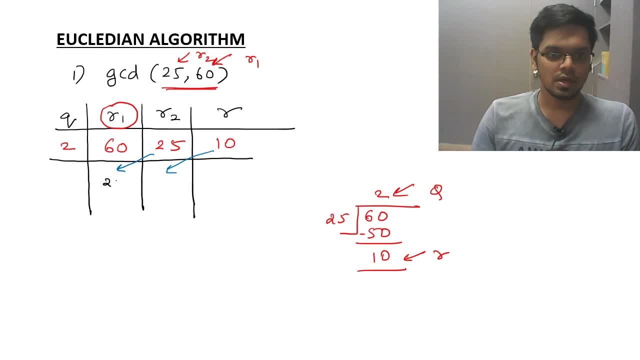 the position. So now the next values are 25, 10.. Again, do the same calculation. What is the calculation? 25.. 25 is divided by 10.. So if you do the calculation, 10, twos are 20 correct and the remainder is 5. So 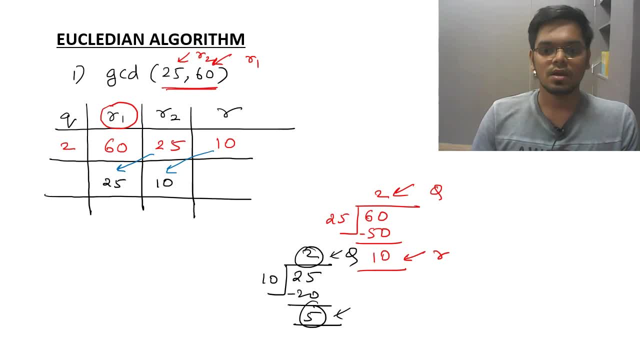 upper part is the coefficient, Lower part is the remainder. So coefficient is 2 and remainder is 5.. So what should be the next step? Come on, Guess the next step and get the answer. The next step is: again we have to do the shifting. This R2 would be at the place of R1.. This R would be at the place. 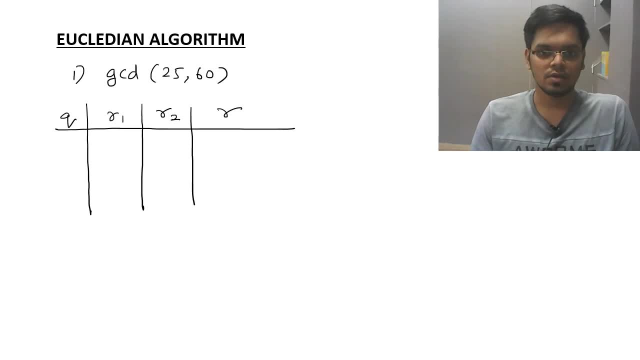 R2.. Column 4: it is the remainder, which is R. So I guess the first step is clear, that is, making the table. We have to write four columns: Column 1 is quotient, Column 2 is row 1.. Column 3 is R2 and column 4 is R. Now, this R1 is the greatest value among these two, Which is: 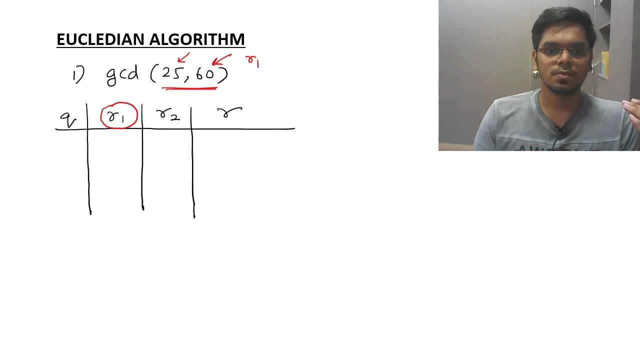 greatest, 60 is greatest right. So this would be R1.. The remaining part would be R2.. So I will write 60 first, then R2. here Now how to find quotient and remainder. It is very simple. Basic calculation: 60 is divided by 25.. So 25 twos are, it would be 50 and remainder would be 10.. So the numerator part. 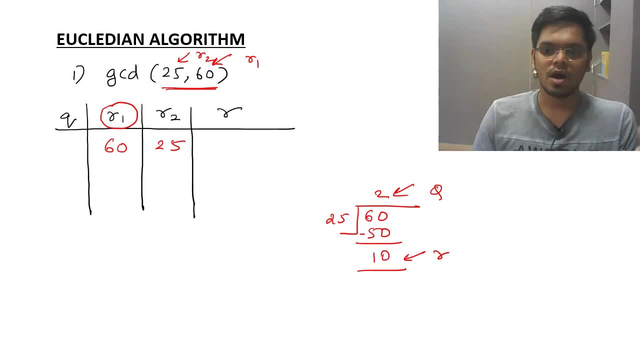 the denominator part is the remainder part. I hope you know how to do the basic division. So quotient is 2.. Remainder is 10.. Now comes the next step, Very important step In the next step: how to get R1 and R2? We have to shift the position. R2 would be here and R would be here. We are shifting. 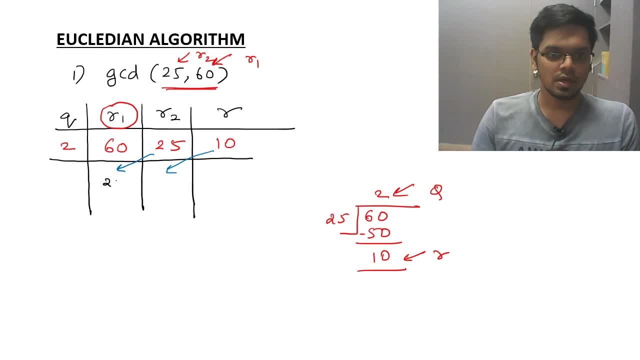 the position. So now the next values are 25, 10.. Again, do the same calculation. What is the calculation? 25.. 25 is divided by 10.. So if you do the calculation, 10, twos are 20 correct and the remainder is 5. So 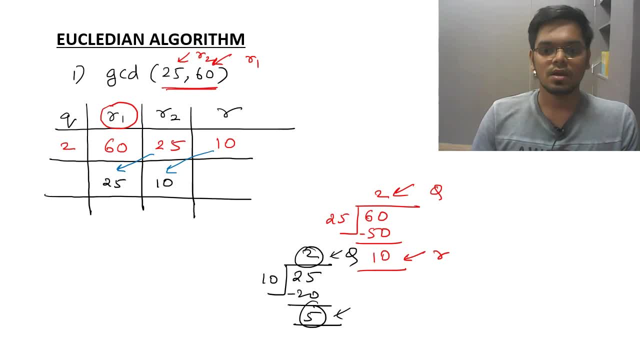 upper part is the coefficient, Lower part is the remainder. So coefficient is 2 and remainder is 5.. So what should be the next step? Come on, Guess the next step and get the answer. The next step is: again we have to do the shifting. This R2 would be at the place of R1.. This R would be at the place. 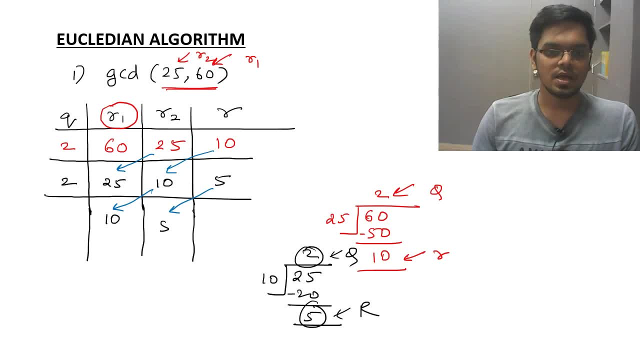 of R2.. So now the calculation is 10, 5.. Again, if you do basic maths. So 10 is divided by 5.. So quotient is 2.. Remainder is 0.. And now again shift the position. So 5 will go here, 0 will go here. Now comes the. 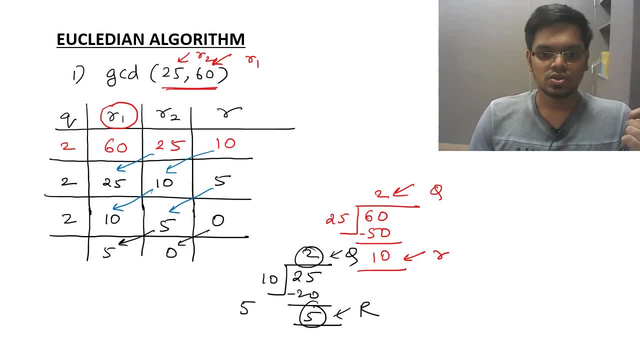 problem. What you are saying is: the 5 is divided by 0, which is not possible. How can you divide 5 over 0?? Is it possible? Answer is no, So you won't get any quotient, You won't get any remainder. And the final? 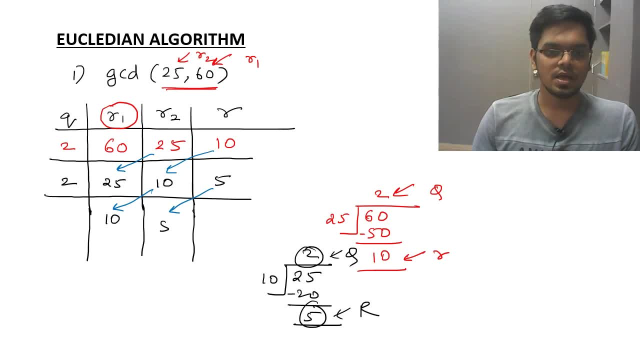 of R2.. So now the calculation is 10, 5.. Again, if you do basic maths. So 10 is divided by 5.. So quotient is 2.. Remainder is 0.. And now again shift the position. So 5 will go here, 0 will go here. Now comes the. 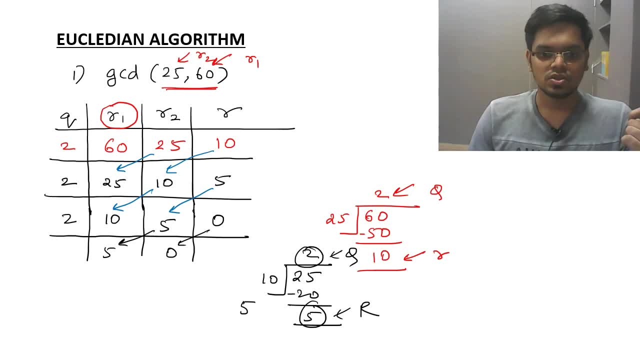 problem. What you are saying is: the 5 is divided by 0, which is not possible. How can you divide 5 over 0?? Is it possible? Answer is no, So you won't get any quotient, You won't get any remainder, And 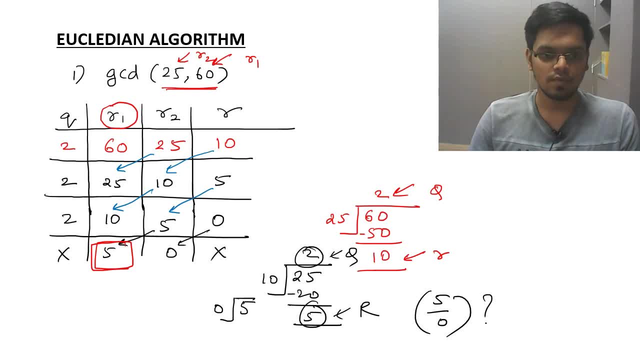 advantage multiple times. So if it depends upon the result of 1 and 0. This is the answer And hilft for solved simple questions. So problem solved is OK Means the final answer is this value. The final answer is R1 value. This is the GCD. GCD is R1 at the end, which is 5.. So this: 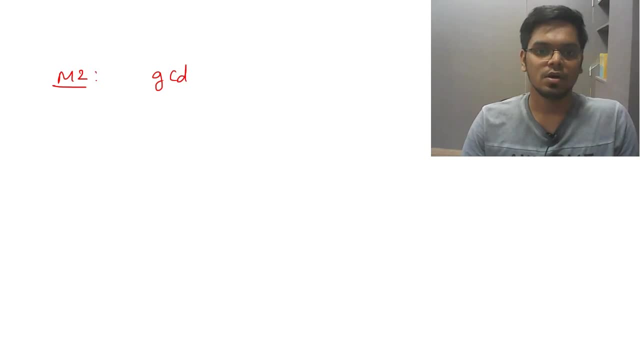 is the algorithm of Euclidean. So let us see method 2: how to solve this question in the fastest way. OK, GCD of 25,60.. Simple: You have to write 25, You have to write 60, right? so 5 5s are 25 and 5 12s are 60, correct? now ask yourself what is common. 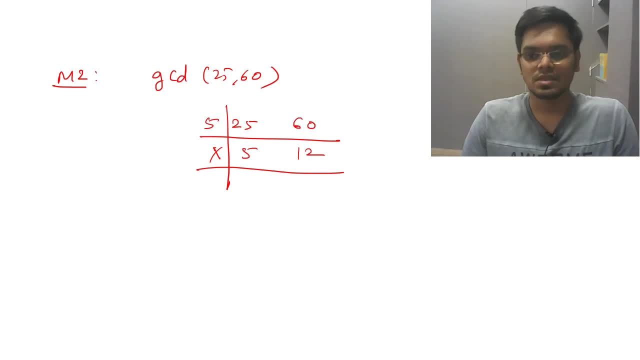 between this two, 5 and 12, nothing is common. this means this is the end of the calculation and whatever is common. that is your answer. this was common, so this is the greatest common divisor, which is equal to 5. that is nothing but GCD of. 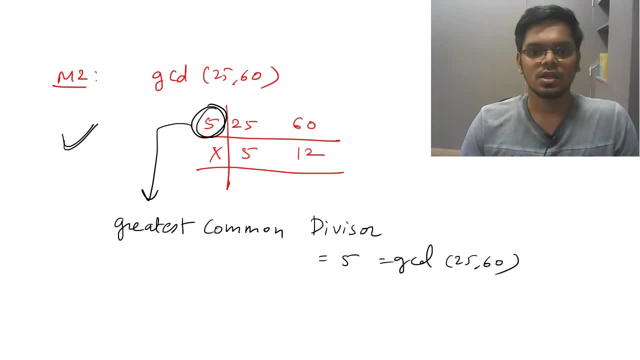 25 comma, 60. okay, you can use this method in your competitive exam. very simple. so I will give you one homework question as well. the homework question is here. do comment what is the answer. this is homework question and you can comment the answer. I will verify whether it is right or not. okay, find a GCD of 60 161. 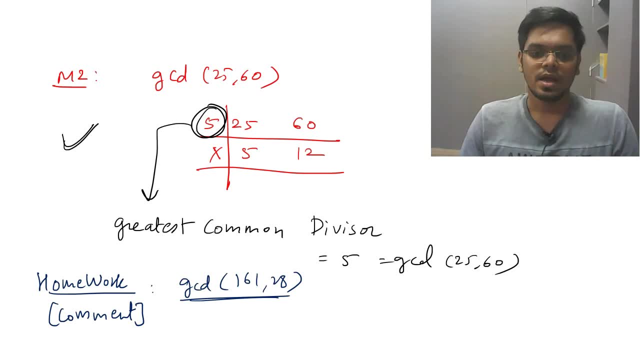 comma 28. okay, so this is the homework question and comment the answer. you can use method 1 or you can use method 2. why I show you method 1? why I show you method 2? why I show you method 1? because if you are writing cryptography, exam cryptography in. 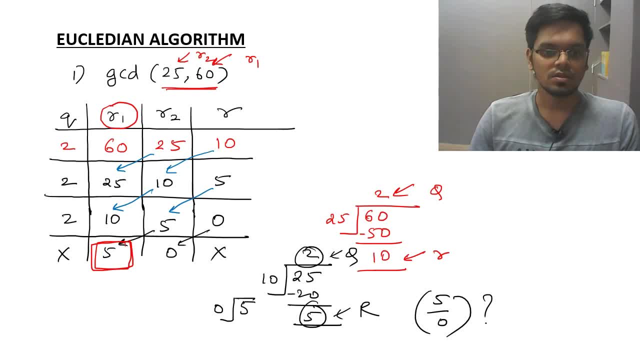 answer is this value. The final answer is the R1 value. This is the gcd. Gcd is R1 at the end, which is 5.. So this is the algorithm of Euclidean. So let us method 2. How to solve this. 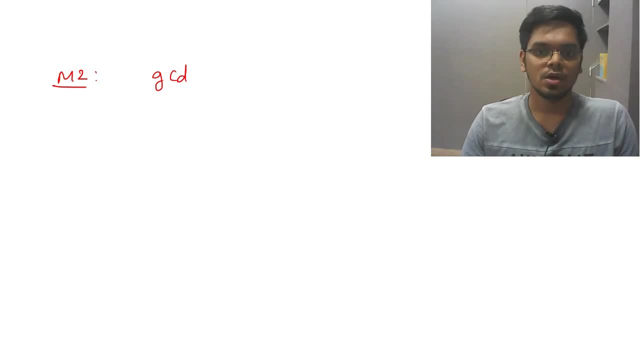 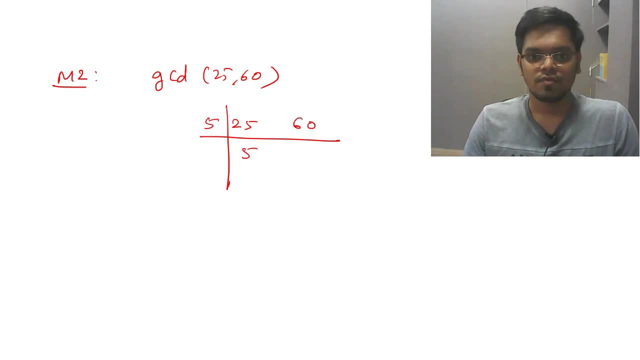 right. So 5 5s are 25 and 5 12s are 60, correct? Now ask yourself what is common between these two 5 and 12?? Nothing is common. This means this is the end of the calculation, and whatever is. 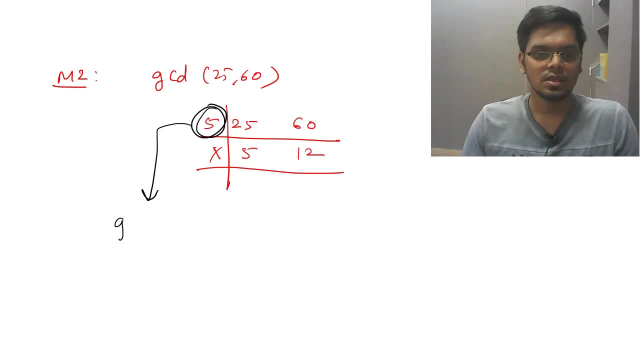 common. that is your answer. This was common. so this is the greatest common divisor, which is equal to 5. that is nothing but GCD of 25 comma 60. You can use this method in your competitive exam. Very simple. So I will give you one homework question as well. The homework question is here. 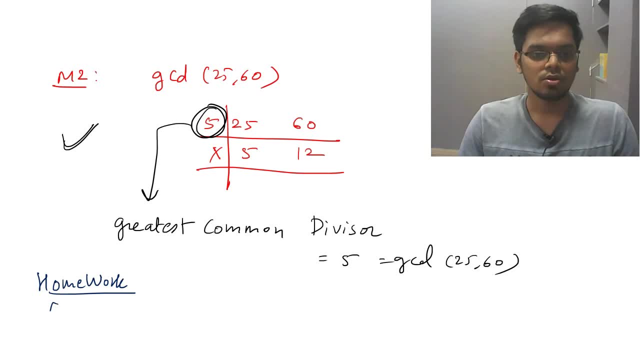 Do comment. what is the answer? This is homework question and you can comment the answer. I will verify whether it is right or not. Find a GCD of 161, comma 28.. So this is the homework question and comment the answer. You can use method 1 or you can use method 2.. Why I showed you method 1? Because if you are writing, 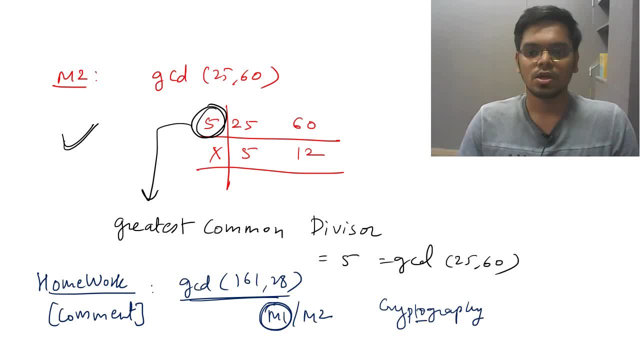 cryptography exam, cryptography in engineering- they will tell you find GCD using the Euclidean algorithm. Then you have to use method 1.. Whereas if you are writing competitive exams, then you can use method 2 to get the answer: Either competitive exam or it can be aptitude exam, or even in the 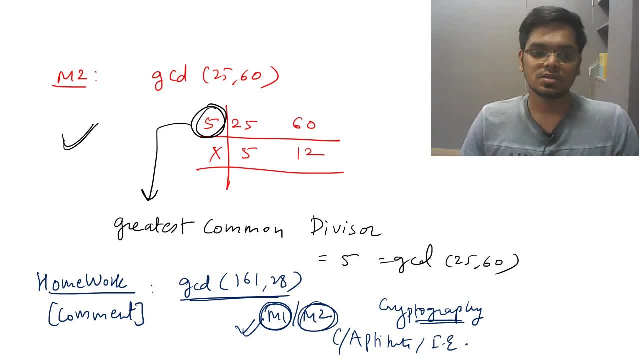 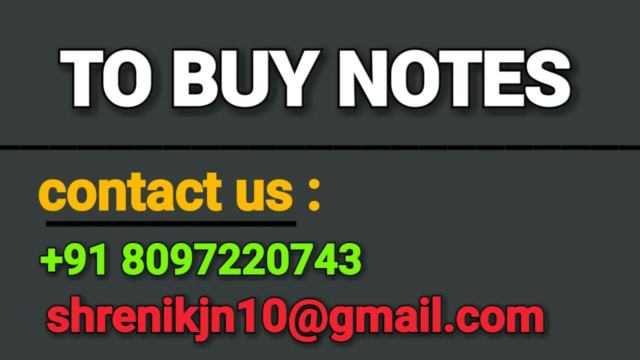 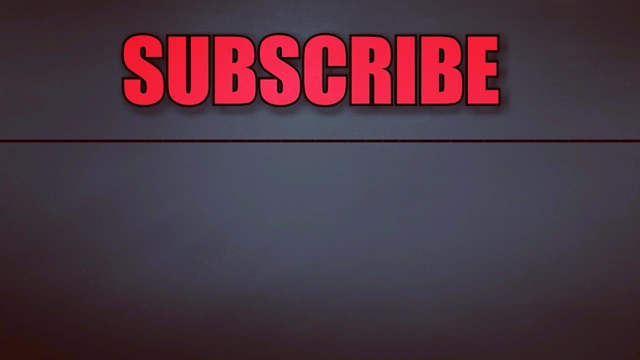 interview exam. So you can use method 2.. So comment the answer and meet in the next video, Take care. So, friends, if you like my video, then do like this video, share with your friends and subscribe to my YouTube channel. So meet you in the next video. Till then, take care. This is Shrenik Jain. Peace out.